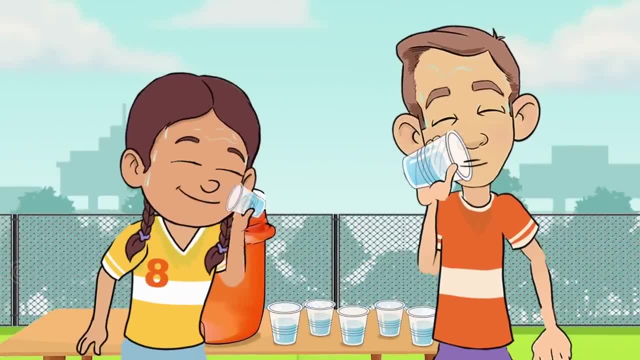 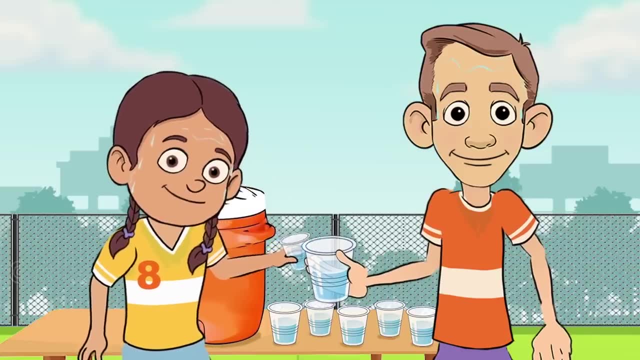 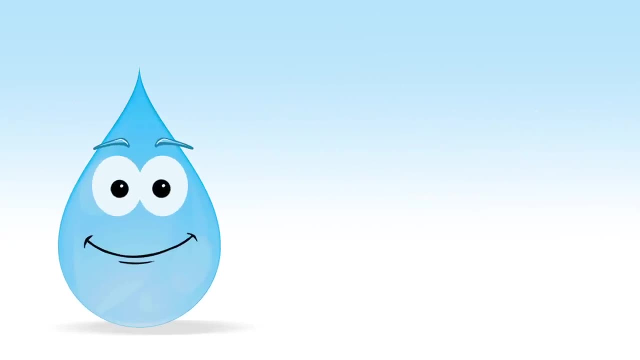 Today, we are going to learn all about the water cycle and how it works, so that we can protect our water and make sure there is plenty for future generations. What is the water cycle? Before we get into the details about this cool process, we need to know what it means. 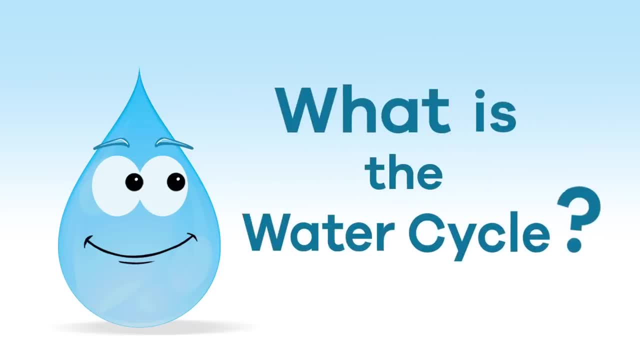 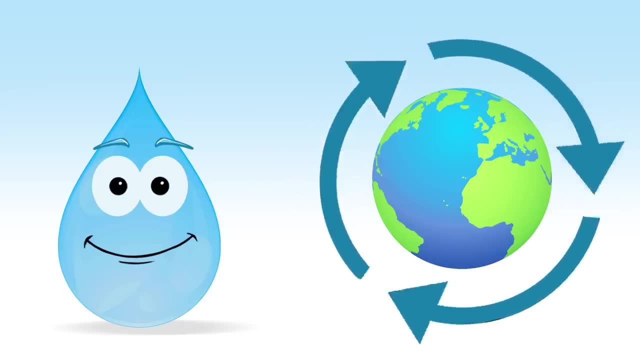 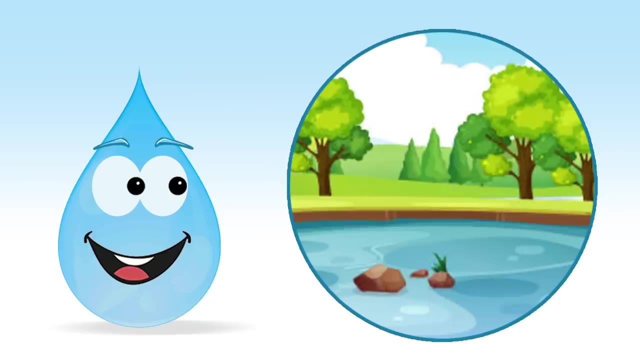 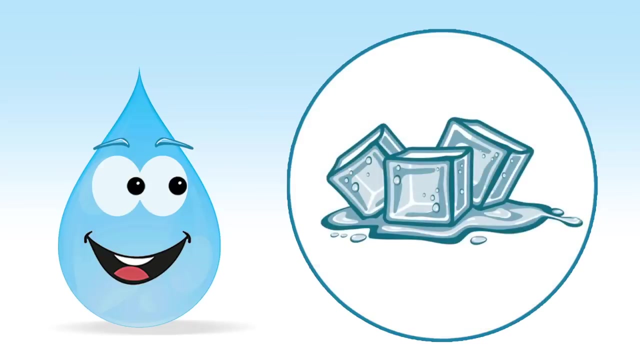 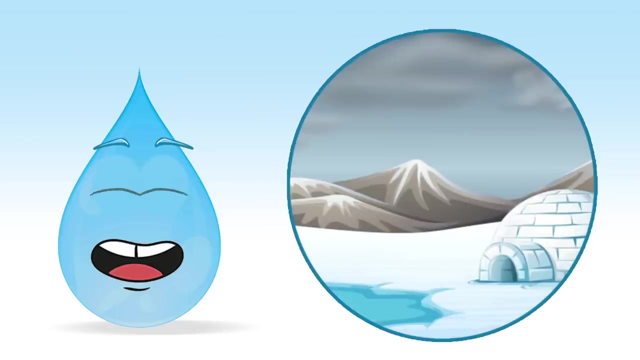 So what is the water cycle? It is the path that all water follows as it moves around the Earth in different states or phases. Water in its liquid phase is found in oceans, rivers, lakes and even underground. Solid water or ice is found in glaciers, snow and at the North and South Poles. 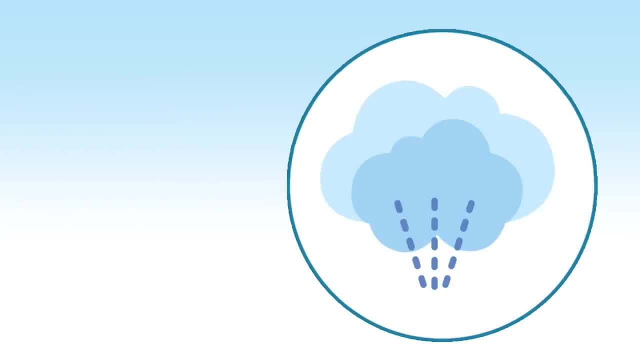 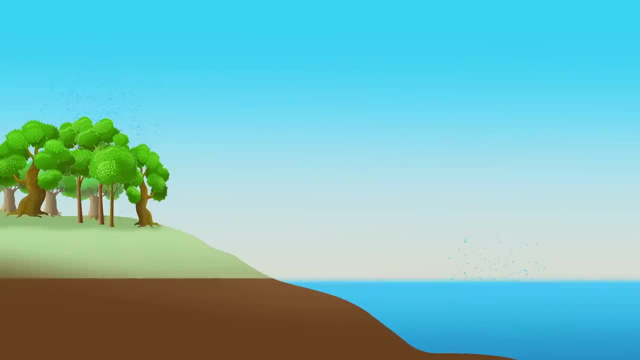 Water vapor is a gas and it is found in the Earth's atmosphere. So what is the water cycle? Water cycle stages. How does this process happen? It happens through four different stages called evaporation, transpiration, condensation and precipitation. 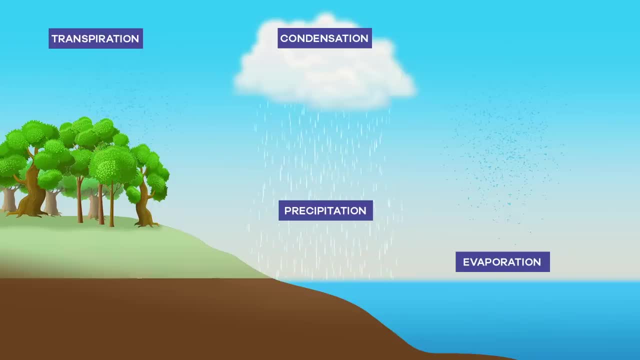 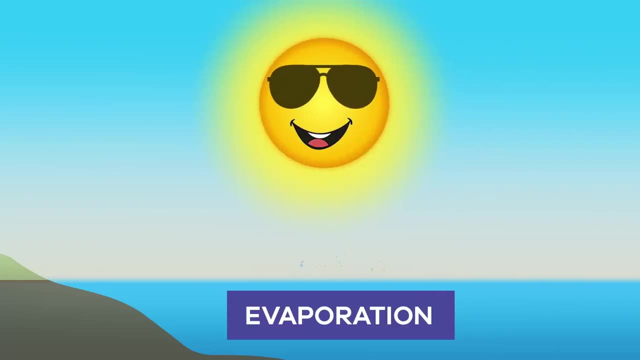 Let's talk about each in more detail. shall we First up evaporation. Evaporation happens when the sun heats up the water, and when the water gets hot enough, it changes into a gas. This gas then evaporates into the air. 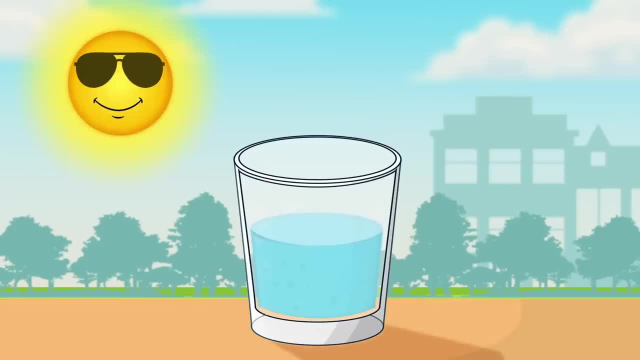 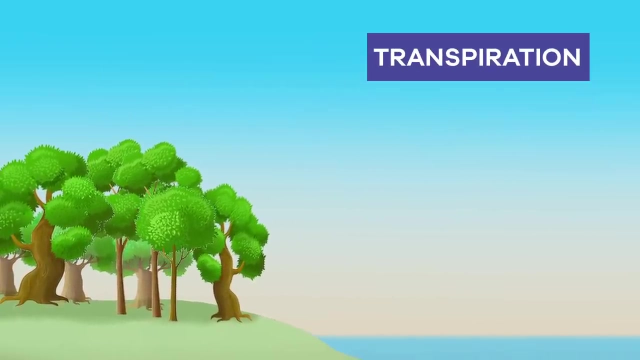 You can see this process for yourself. if you leave an open container of water in your home or outside, Once it gets hot enough, it will evaporate. Next up: transpiration. Transpiration is the process by which plants lose water in the form of water vapor. 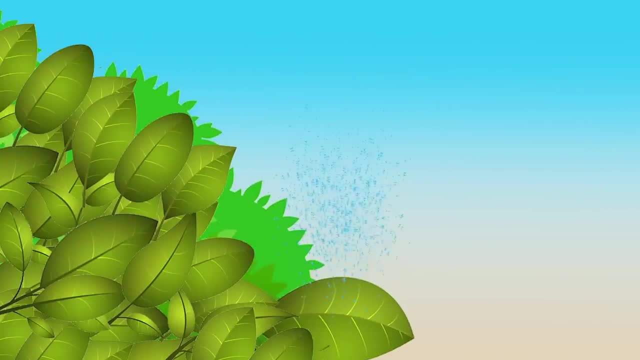 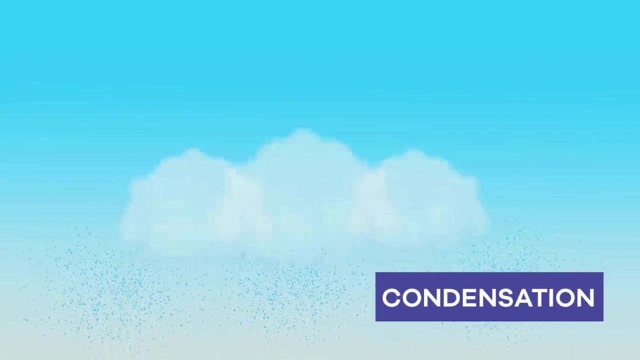 Basically, it is the release of water through a plant's leaves and is similar to evaporation, because that water vapor goes into the air. Condensation- Condensation occurs when the water vapor goes into the air. The water vapor in the air becomes cold and changes back into a liquid. 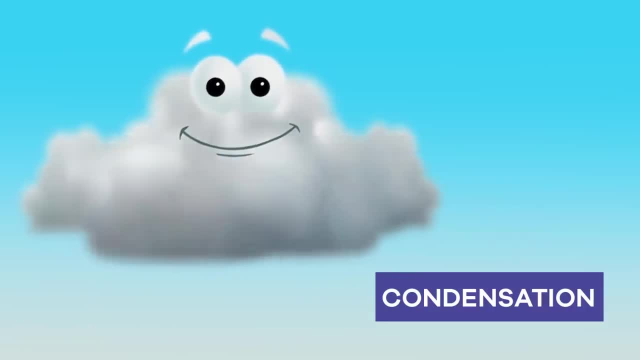 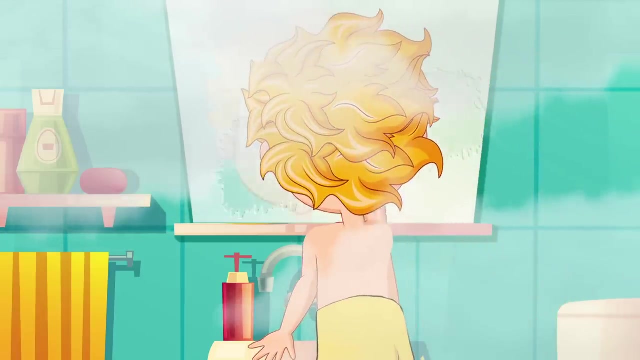 This is how clouds are formed. Can you guess what happens when there is too much moisture in a cloud? It rains, And if you want to see condensation as it is happening, look at your bathroom mirror after you have taken a hot shower. 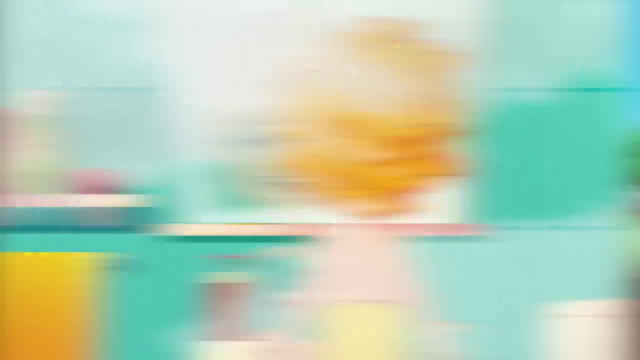 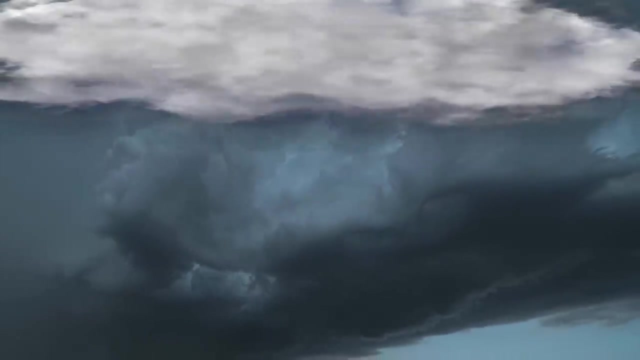 You will see lots of condensation. Finally, evaporation: Precipitation. Precipitation is rain, snow, sleet or hail that falls to the ground, And it happens when the air can no longer hold the water that has been evaporated. 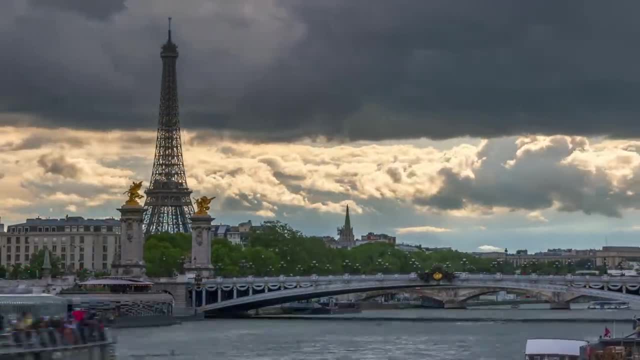 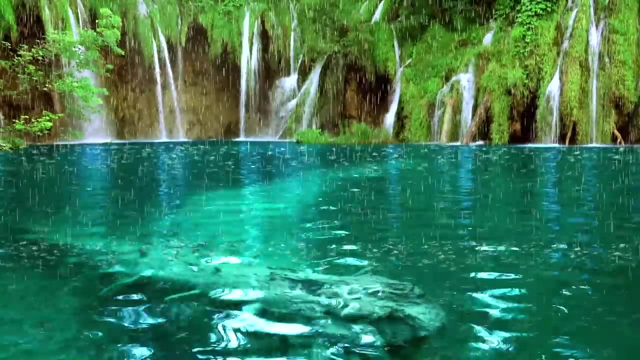 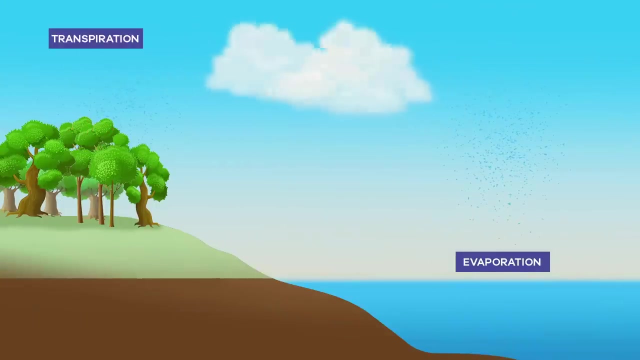 As we mentioned before, when clouds get too heavy, it rains And the evaporated water makes its way back down to the earth. This precipitation will gather in bodies of water or underground And the whole water cycle starts again, Since we have a limited amount of water on our planet. 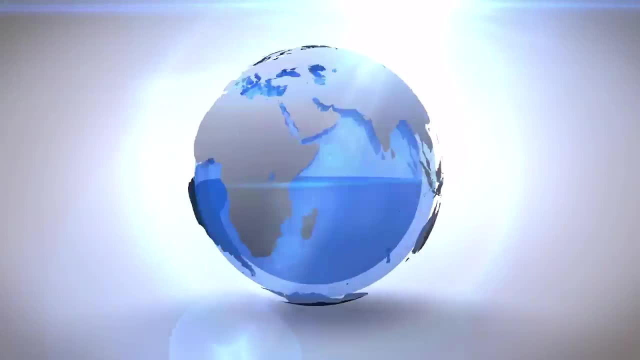 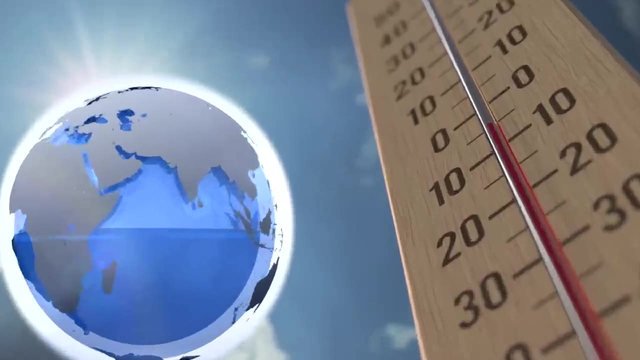 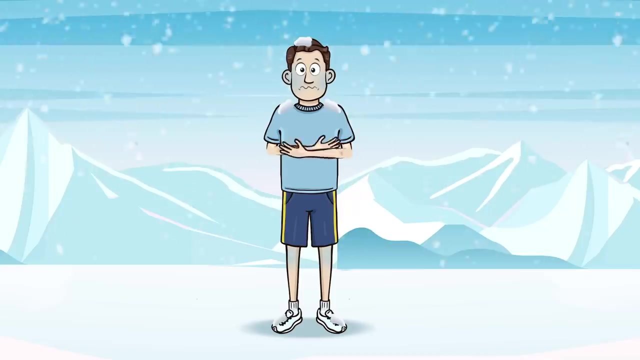 it is important to take care of it. Here is an interesting fact: The water cycle is critical to maintaining and determining the earth's temperature. Without it, the earth's temperature becomes extremely hot or extremely cold, which has a huge impact on both plant and animal life. 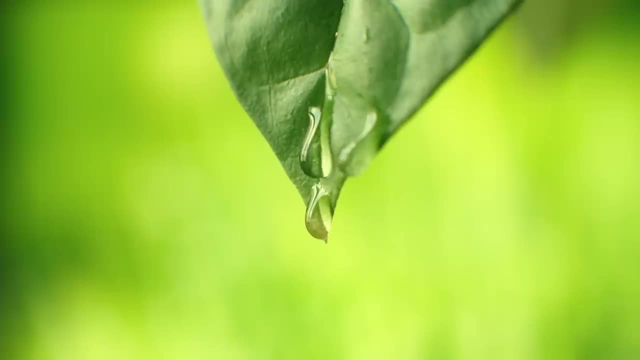 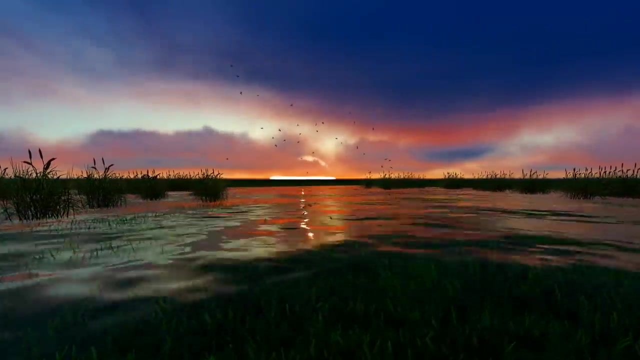 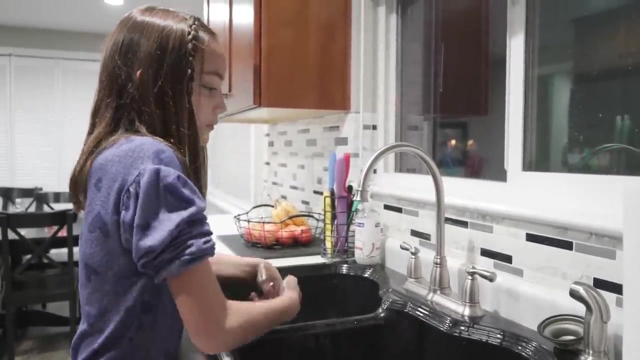 Knowing how the water cycle works and how humans can protect it is very important to the future survival of the planet. So how can you help? Well, one of the best things you can do is to conserve water whenever you can, Whether that means turning off the faucet when you're brushing your teeth. 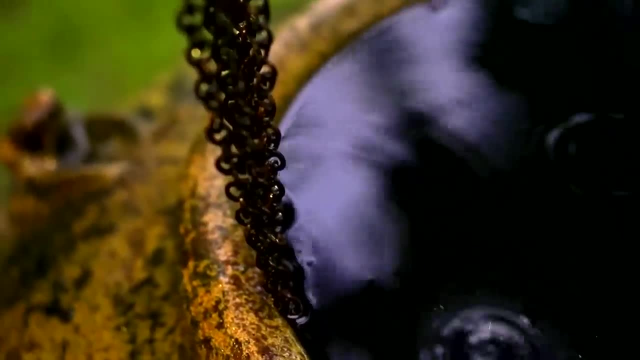 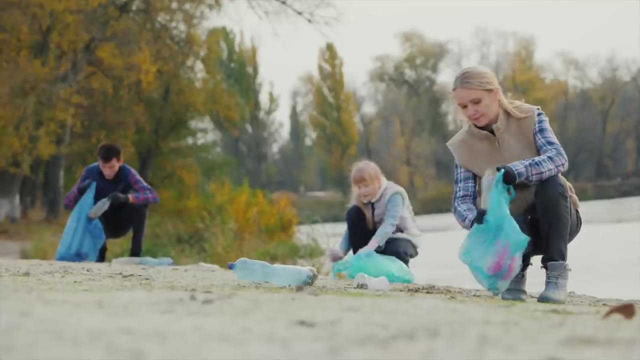 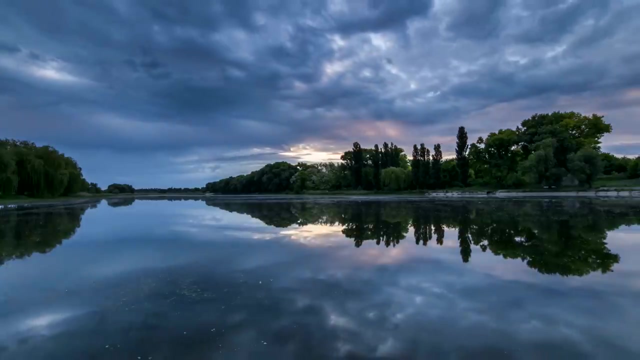 or taking a shorter shower. every little bit helps. You can also talk to your parents about watering your lawn less during hotter months. Another way to protect the water is to keep it clean, which means no littering, especially in your local lakes, rivers and streams.